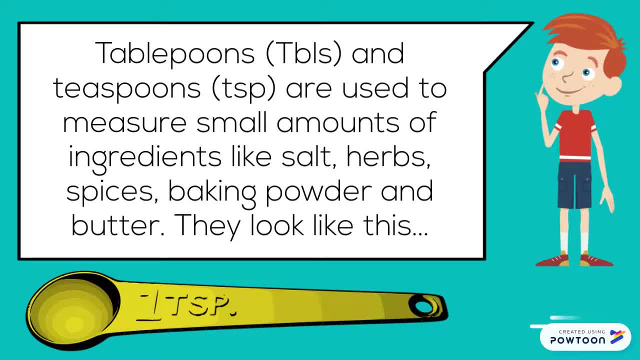 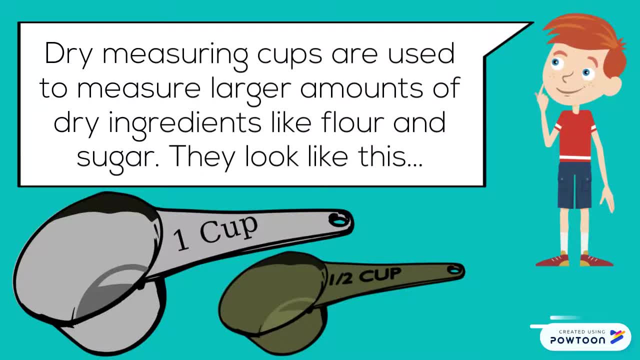 Tablespoons and teaspoons are used to measure small amounts of ingredients like salt, herbs, spices, baking powder and butter. They look like this. Dry measuring cups are used to measure larger amounts of dry ingredients like flour and sugar. They look like this. 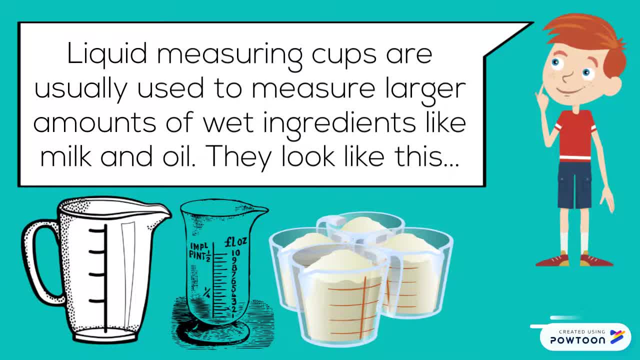 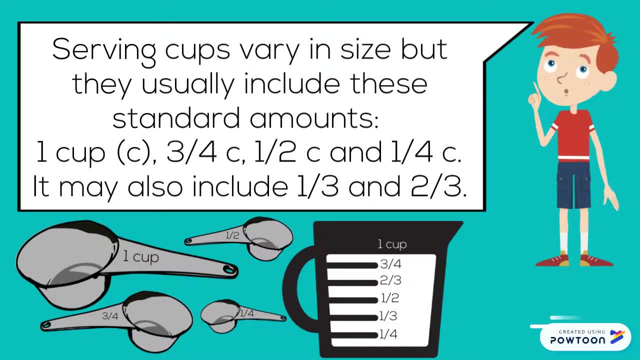 Liquid measuring cups are usually used to measure larger amounts of wet ingredients like milk and oil. They look like this: Serving cups vary in size, but they usually include these standard amounts: One cup, three-quarter cup, one-half cup and one-quarter cup. 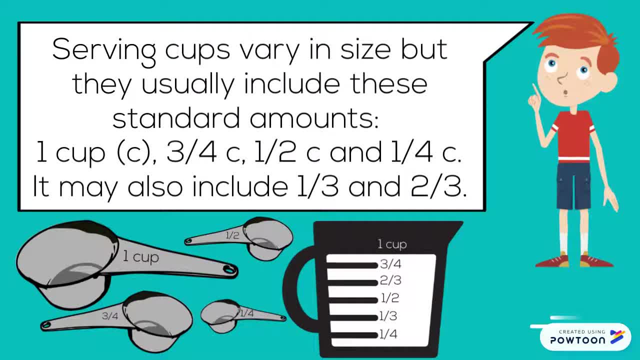 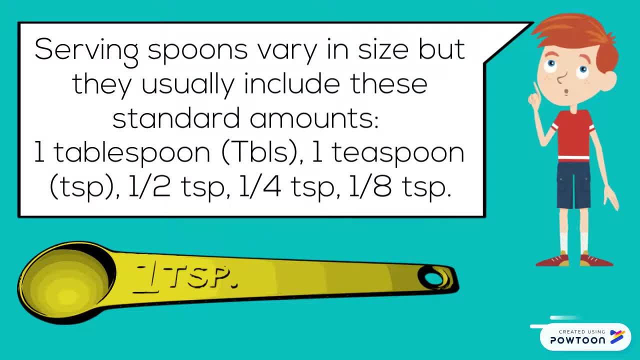 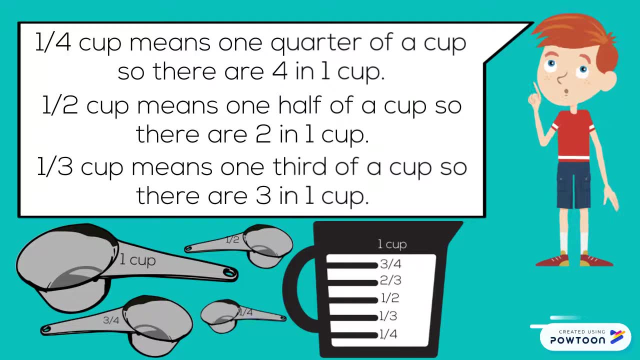 It may also include one-third cup and two-thirds cup. Serving spoons vary in size, but they usually include these standard amounts: One tablespoon, one teaspoon, one-half teaspoon, one-quarter teaspoon and one-eighth teaspoon. One-quarter cup means one-quarter of a cup, so there are four in one cup. 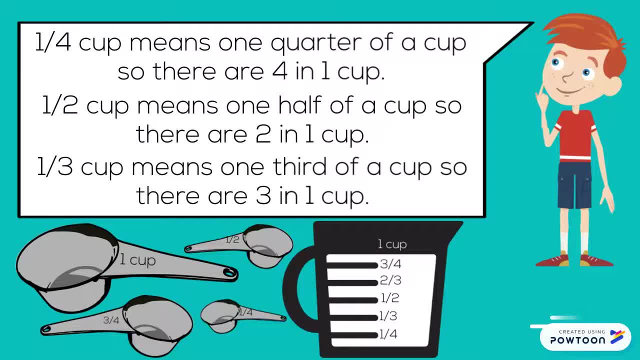 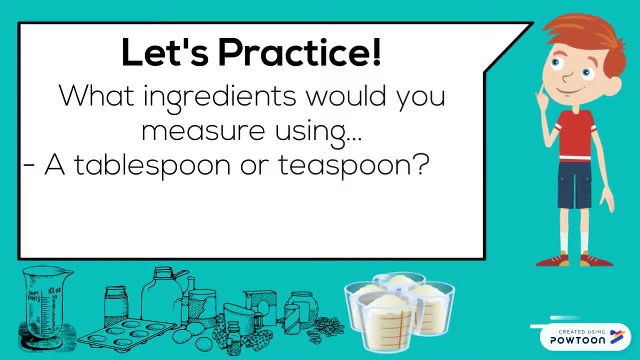 One-half cup means one-half of a cup, so there are two in one cup. One-third cup means one-third of a cup, so there are three in one cup. Let's practice. What ingredients would you measure using a tablespoon or teaspoon? 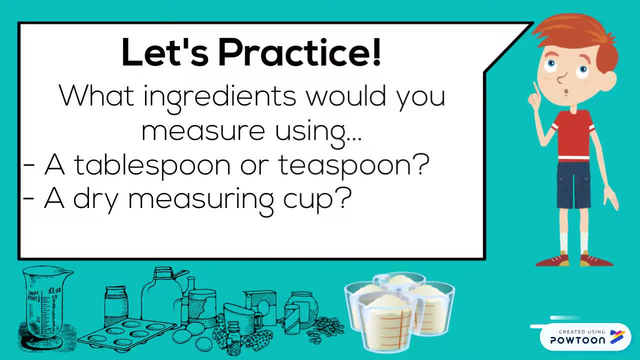 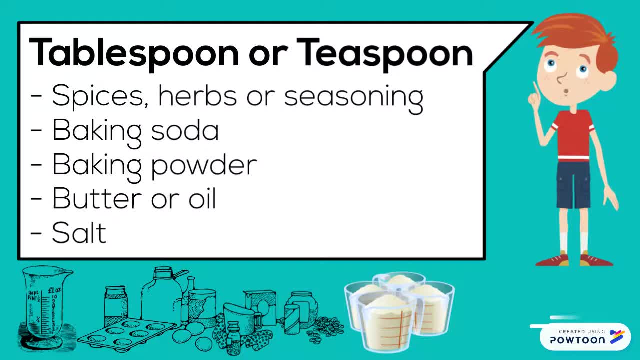 A dry measuring cup, A liquid measuring cup, Tablespoon or teaspoon measures spices, herbs, seasoning, baking soda, baking powder, butter, oil and salt. Dry measuring cups measure flour, sugar, cocoa powder, chocolate chips, walnuts, fruit and milk. 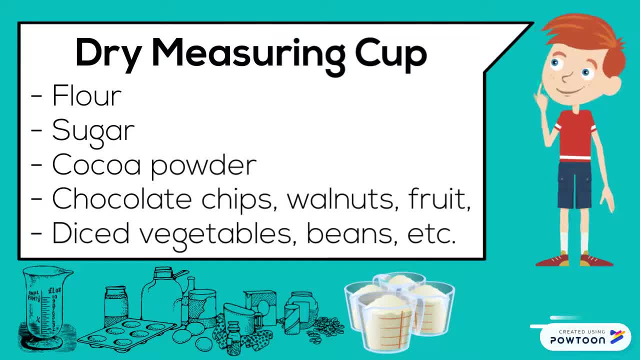 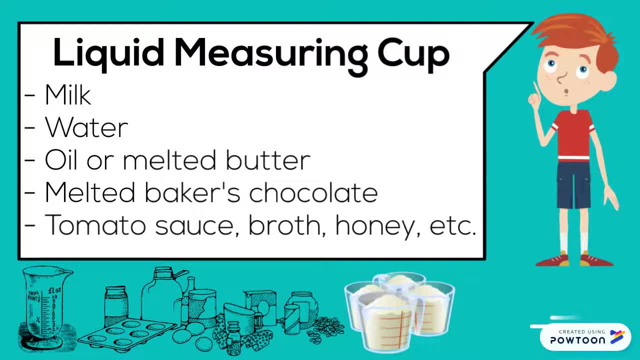 Dry measuring cups measure flour, sugar, cocoa powder, chocolate chips, walnuts, fruit, milk and salt, Diced vegetables, beans etc. Diced vegetables, beans etc. Liquid measuring cup measures milk, water, oil, melted butter, melted baker's chocolate, tomato sauce, broth, honey, etc. 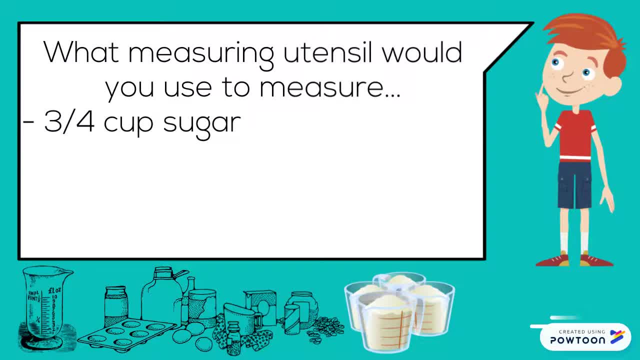 What measuring utensil would you use to measure three-quarter cup sugar? What measuring utensil would you use to measure three-quarter cup sugar? Two-third cup milk. Two-third cup milk. Two tablespoons honey. Two tablespoons honey. One-quarter teaspoon salt. 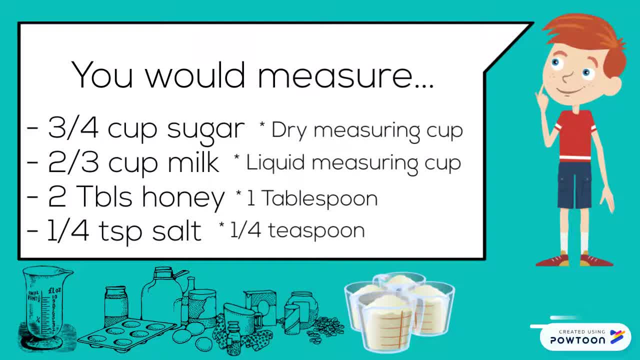 One-quarter teaspoon salt. You would measure three-quarter cup sugar with a dry measuring cup. Two-third cup milk with a liquid measuring cup. Two tablespoons honey with one tablespoon. One-quarter teaspoon salt with a quarter teaspoon. Sometimes, when baking, you might want to make double or half the recipe for more or fewer people. 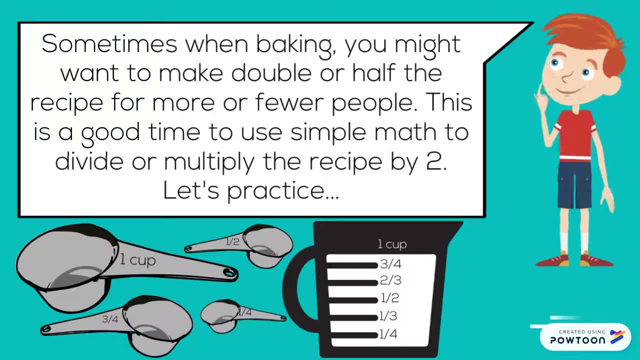 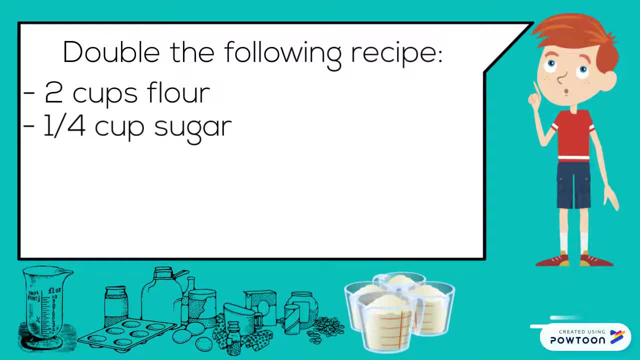 This is a good time to use simple math to divide or multiply the recipe by two. Let's practice Double the following recipe: Two cups flour, one-quarter cup sugar, one-third cup milk, two-thirds tablespoon honey, three-quarter teaspoon salt. 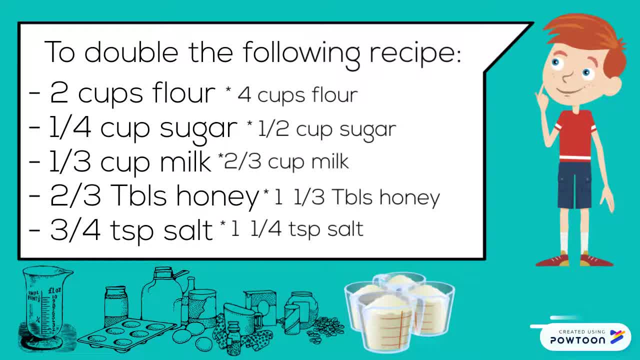 To double the following recipe: two cups flour becomes four cups flour. One-quarter cup sugar becomes a half cup sugar. One-third cup milk becomes two-thirds cup milk. Two-thirds tablespoon honey becomes one and one-third tablespoon honey and one third tablespoon honey. and three quarter teaspoon salt becomes one and one quarter teaspoon. 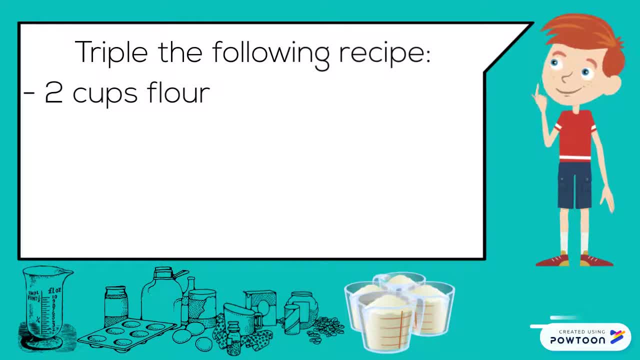 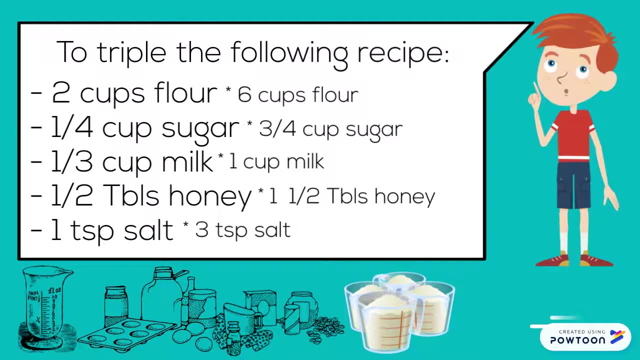 salt, triple the following recipe: two cups flour, one quarter cup sugar, one third cup milk, a half tablespoon honey, one teaspoon salt. to triple the following recipe: two cups flour becomes six cups flour. one quarter cup sugar becomes three quarters cup sugar. one third cup milk becomes one cup milk. one half tablespoon honey becomes one and one half tablespoon honey. 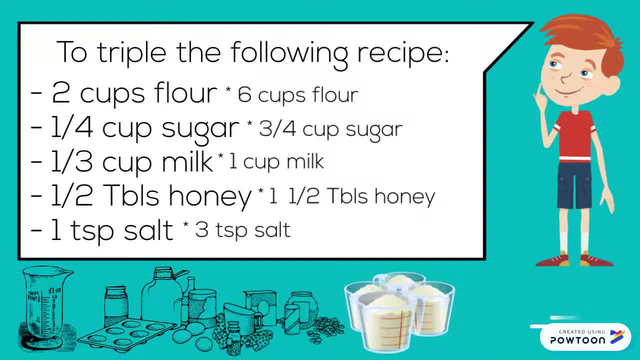 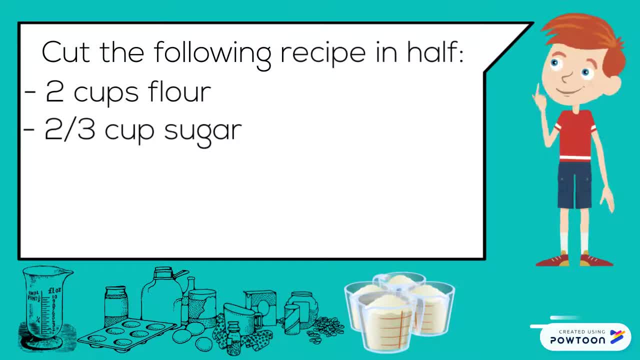 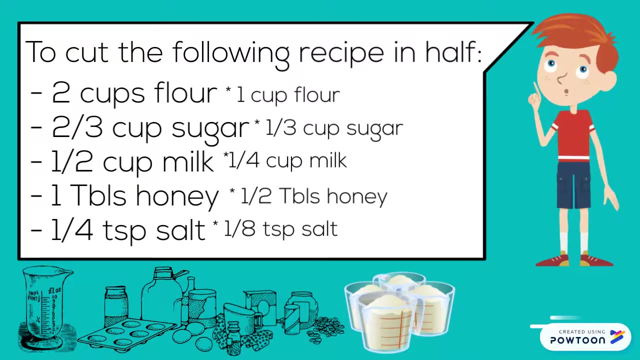 and one teaspoon salt becomes three teaspoons. cut the thong recipe in half: two cups flour, two thirds cup sugar, one half cup milk, one tablespoon honey, one quarter teaspoon salt. to cut the following recipe in half: two cups flour becomes one cup flour. two thirds cup sugar becomes one third cup sugar. one half cup milk becomes one quarter cup milk. 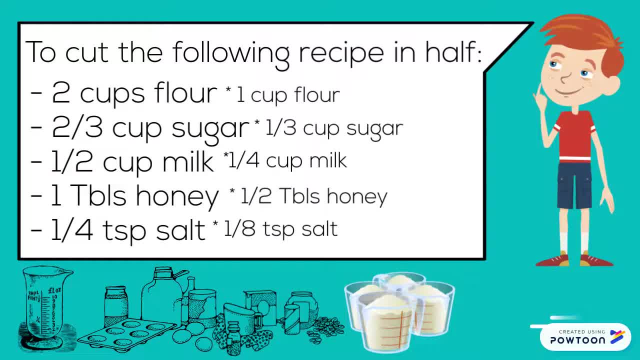 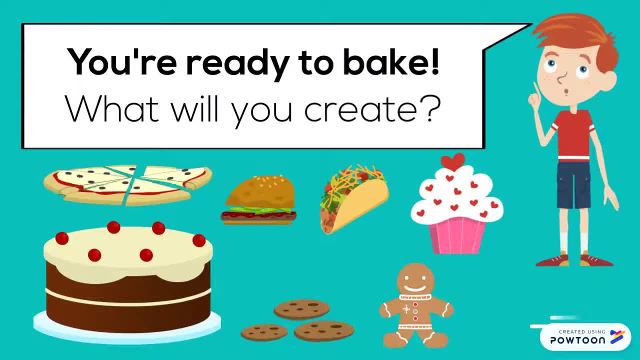 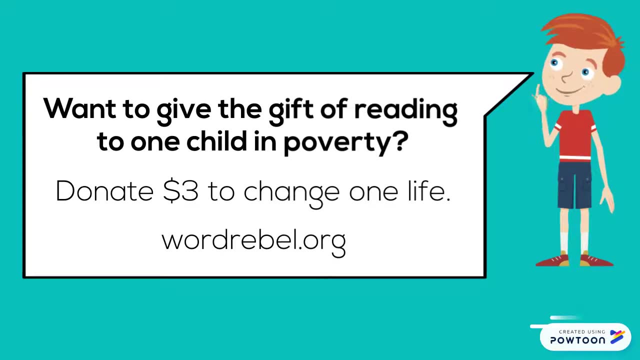 one tablespoon honey becomes one half tablespoon honey and one quarter teaspoon salt becomes one eighth teaspoon salt. you're ready to bake. what will you create? want to give the gift of reading to one child in poverty? donate three dollars to change one life. visit wordrebelorg.